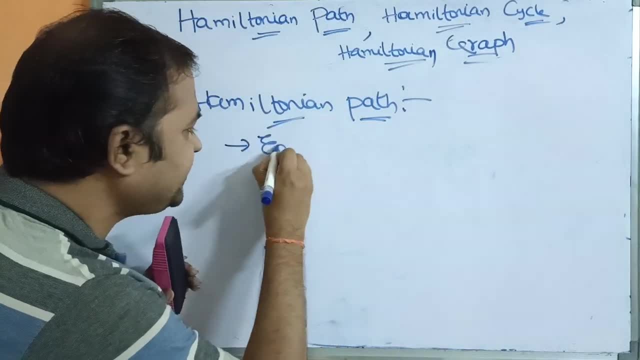 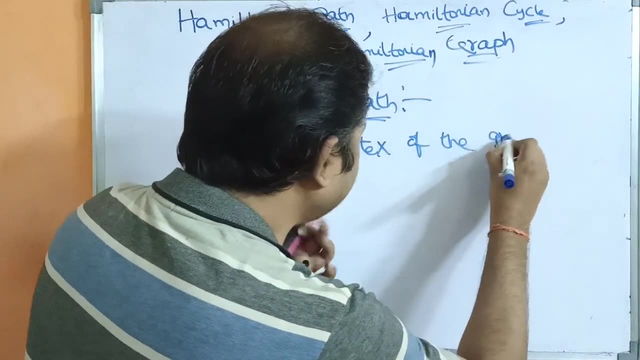 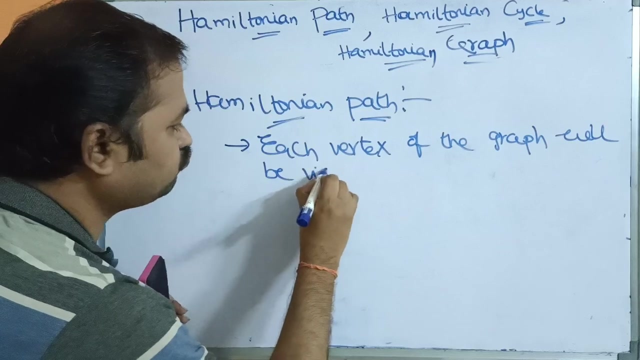 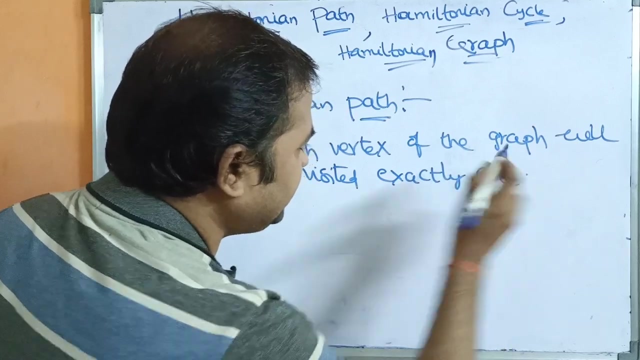 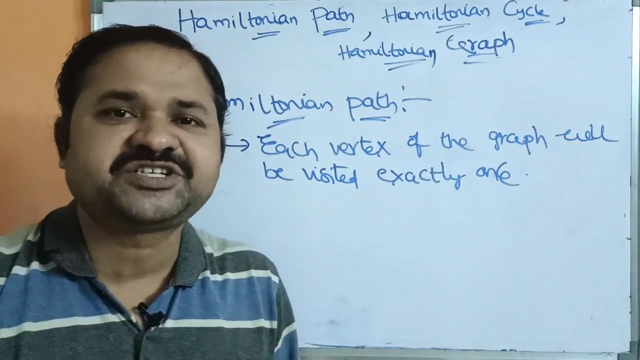 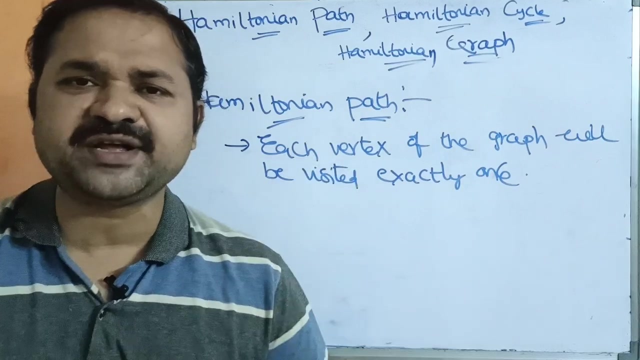 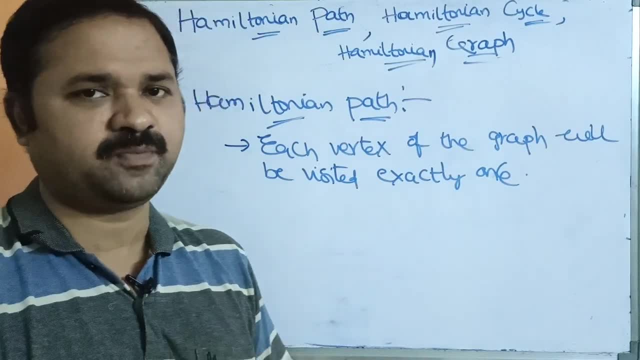 Or if 2,, 3 or 4 edges are not covered, there is no problem. Or if 2,, 3 or 4 edges are not covered, there is no problem. Or if 2,, 3 or 4 edges are not covered, there is no problem. 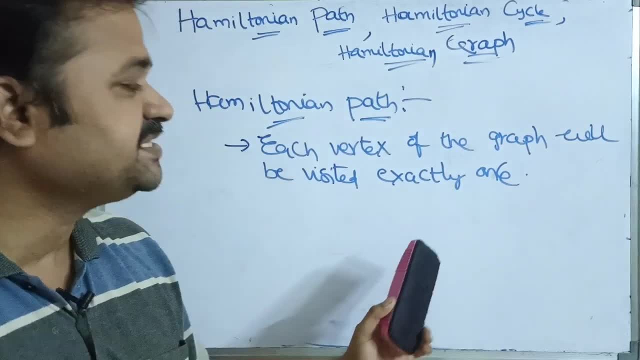 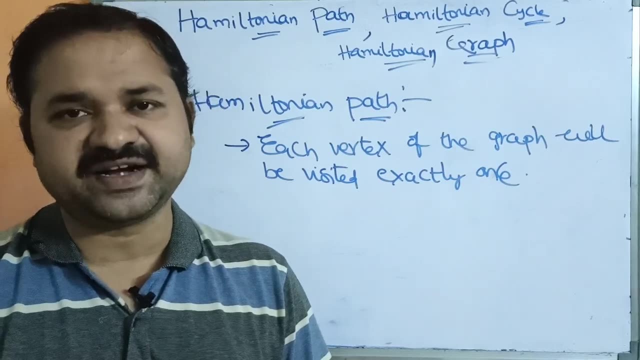 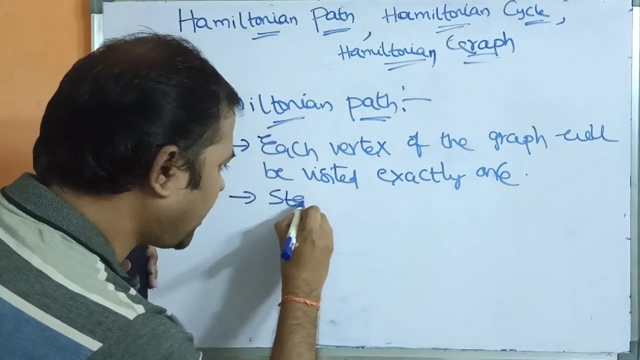 But each vertex of the graph will be visited exactly once. If a graph contains 10 vertices, then we have to visit all the 10 vertices exactly once. So we know what is a path here. Hamiltonian path means start and end vertex must be different. 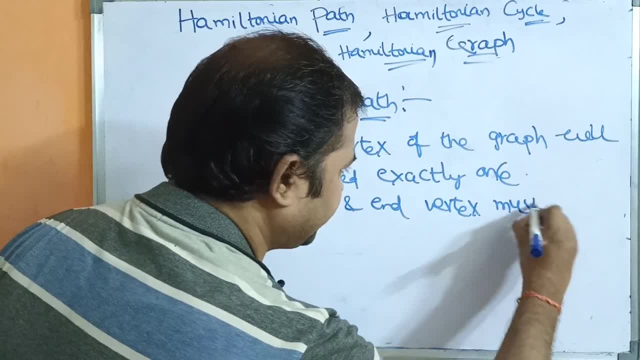 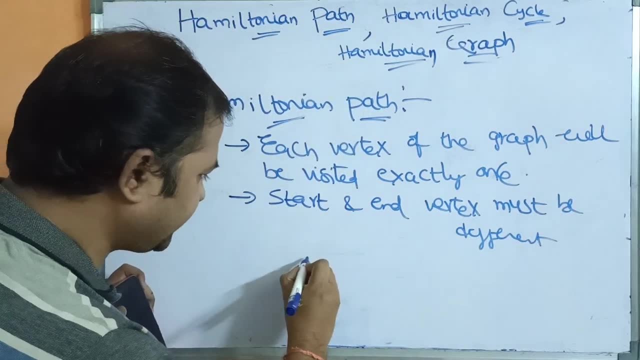 Start and end vertex must be different, Must be different, Must be different Example. Let's take an example here: A, B, C, D. Let we have a path like this: A, B, C, D, E. 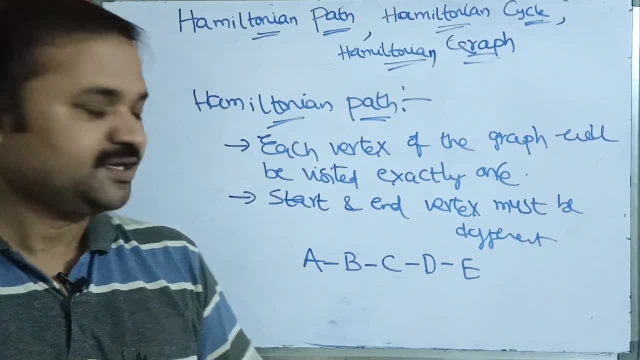 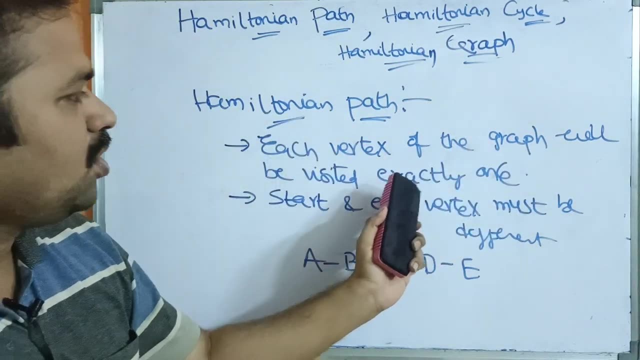 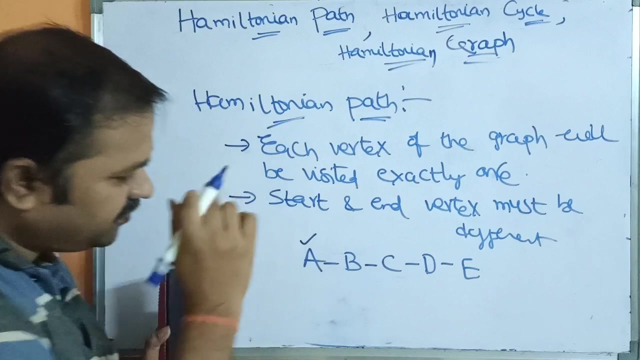 Let a graph contains totally 5 vertices, Then let us assume that this is the path. Why? Because we know that here we have to visit all the vertices of the graph exactly once. Here in this path, it is starting, Starting at vertex A. 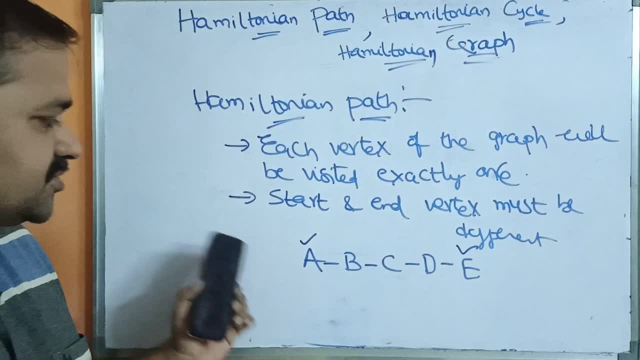 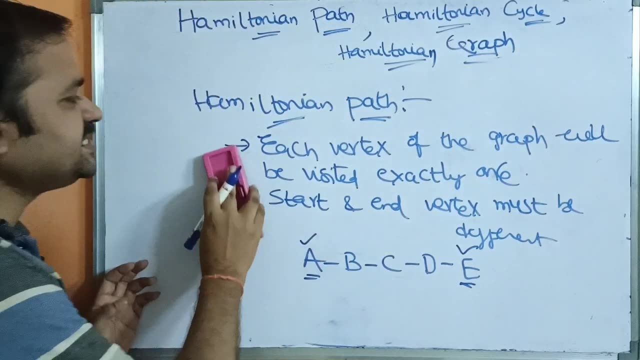 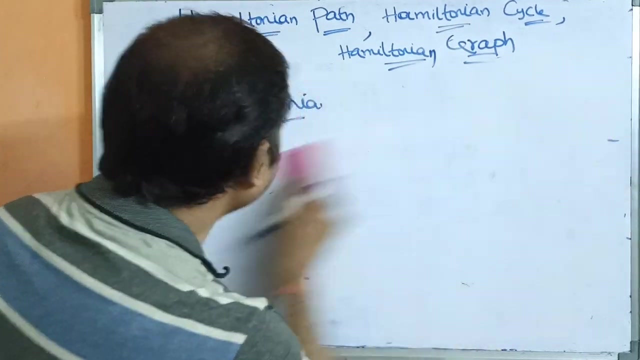 And what is the ending vertex? Ending vertex is E, So starting vertex and ending vertex are different. So this is about Hamiltonian path. Now let us see about Hamiltonian cycle, Hamiltonian cycle. Hamiltonian cycle can also be called as Hamiltonian circuit. 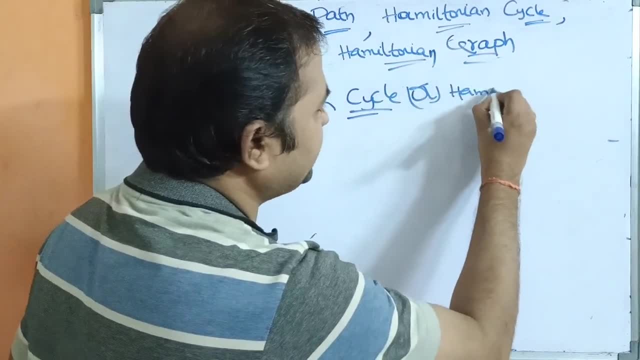 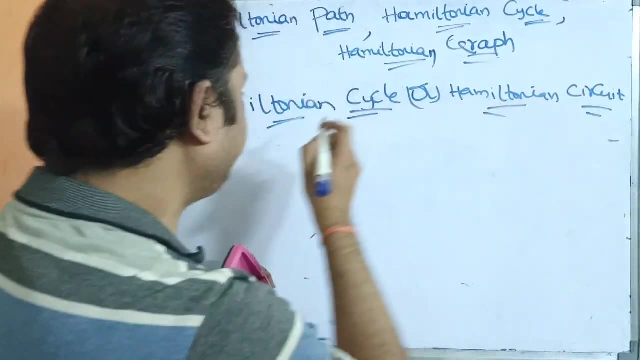 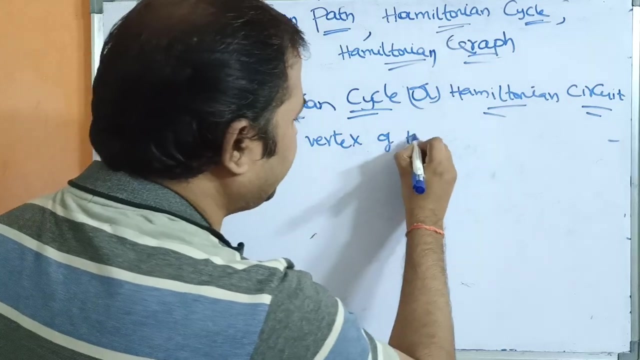 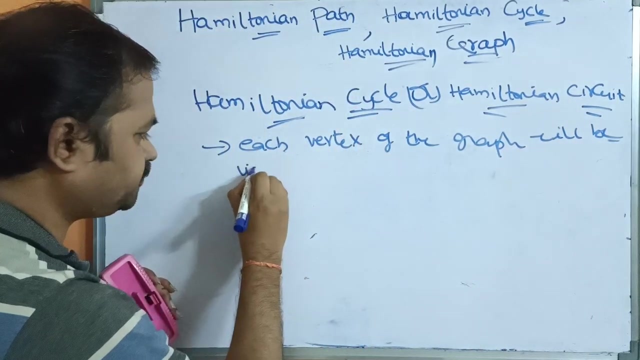 Hamiltonian cycle or Hamiltonian circuit, Hamiltonian circuit. So both are same, only, Both are same only. Let us see what is Hamiltonian circuit. So here also, each vertex of the graph, Each vertex of the graph will be visited. Each vertex of the graph will be visited, exactly once. 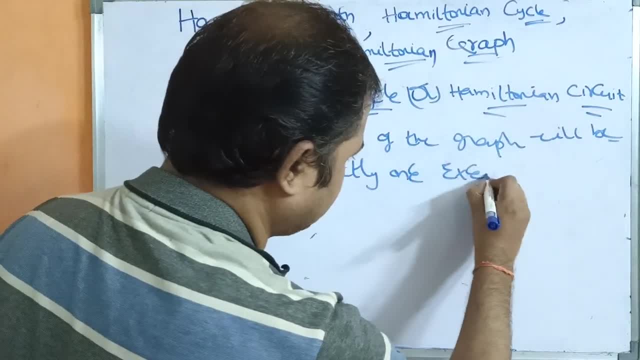 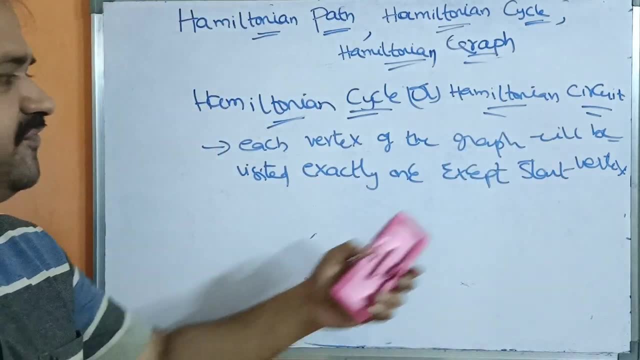 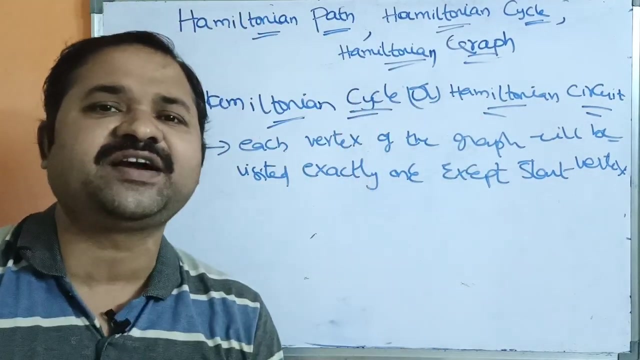 Except start vertex. Except start vertex, Each vertex of a graph will be repeated, Will be visited exactly once, Except the start vertex. Why? Because here the start vertex and end vertex must be the same. Let here the path, this cycle. 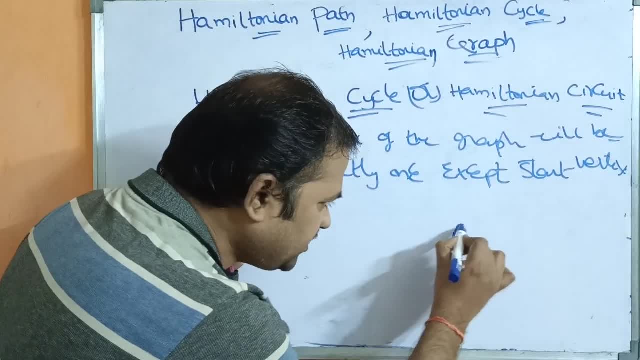 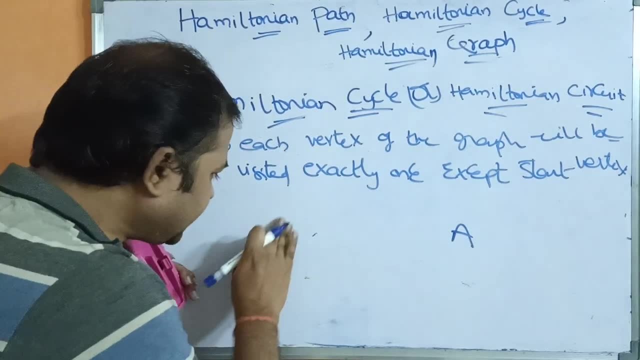 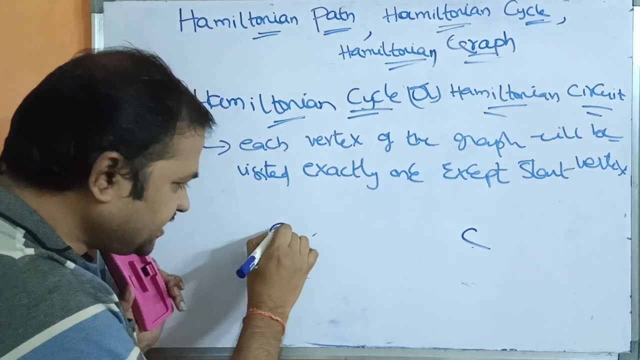 It is starting at the vertex A, Then it also ends at the vertex A. So that means, here the start vertex must be repeated. Okay, Let the cycle starts at the vertex A, Then it should end at C. Let the circuit starts at vertex C. 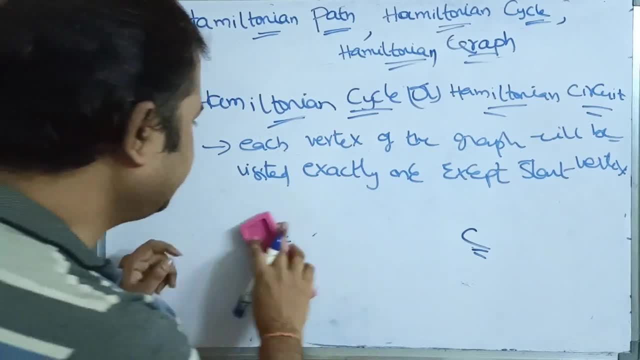 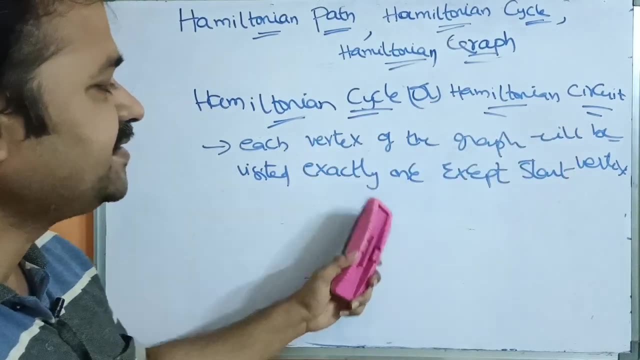 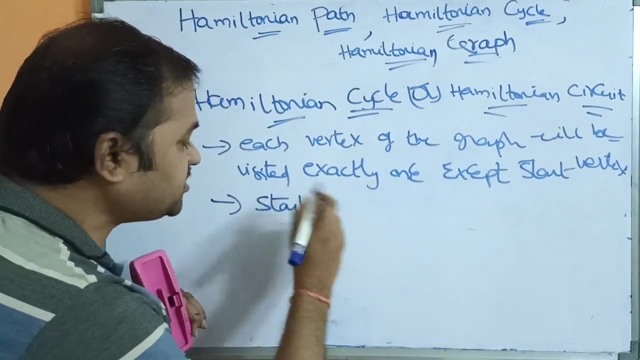 Then it should end at the vertex C. Okay, So this is about what is Hamiltonian cycle or circuit. Each vertex of the graph will be visited exactly once, Except start vertex. That means here start vertex and end vertex must be same- Start and end. 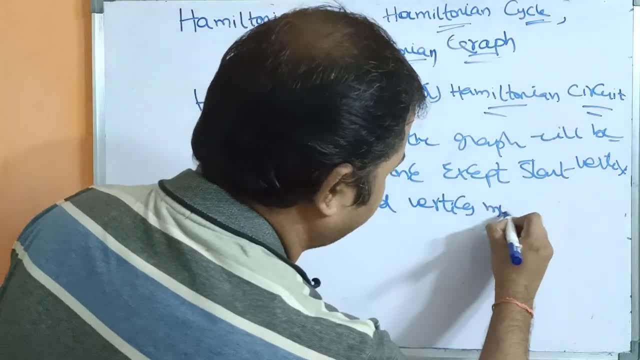 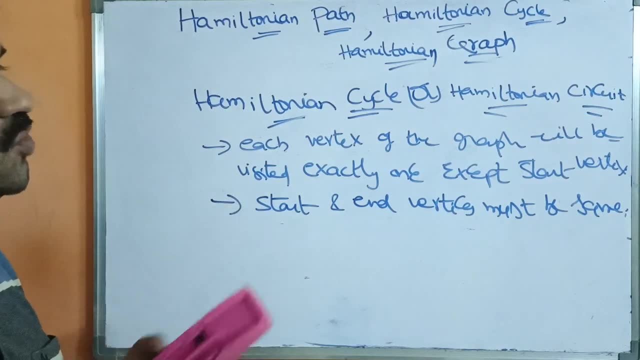 And end vertices must be same, Must be same, So we can repeat the start vertex, But no other vertex can't be repeated. Okay, This is about what is Hamiltonian cycle or what is Hamiltonian circuit, And the next terminology is Hamiltonian graph. 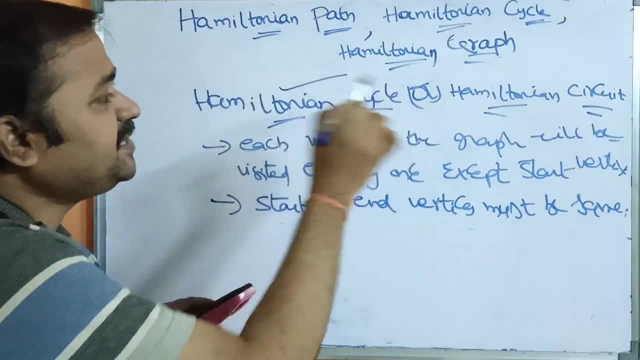 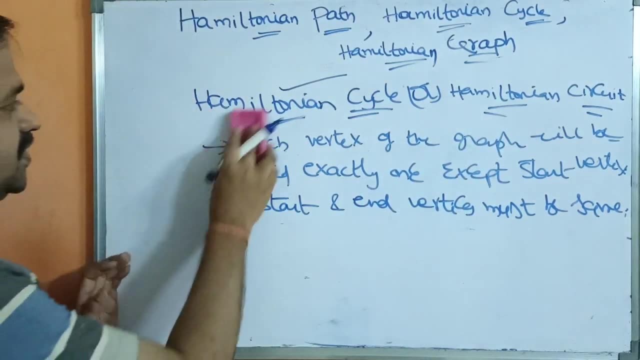 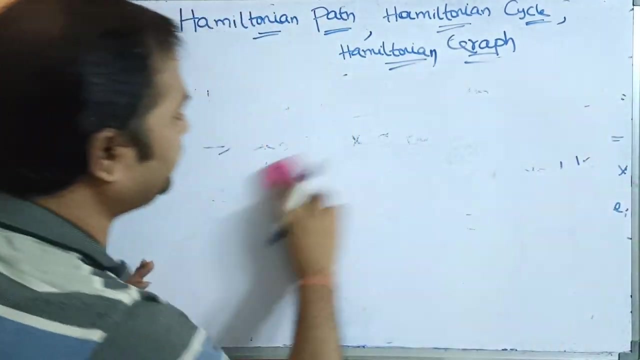 Hamiltonian graph means: if the graph contain Hamiltonian cycle or Hamiltonian circuit, Then the corresponding graph is called as Hamiltonian graph. So what is Hamiltonian graph? If the graph contains Hamiltonian cycle or circuit, then the corresponding graph is called as Hamiltonian graph. 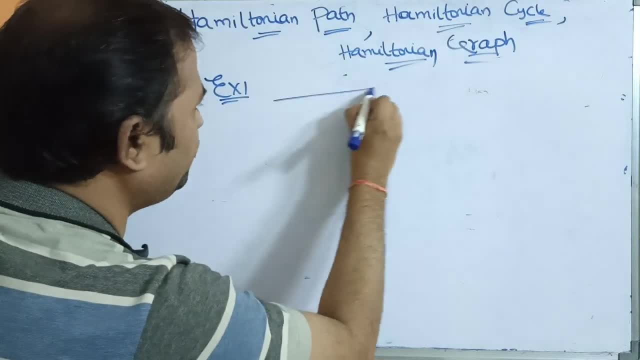 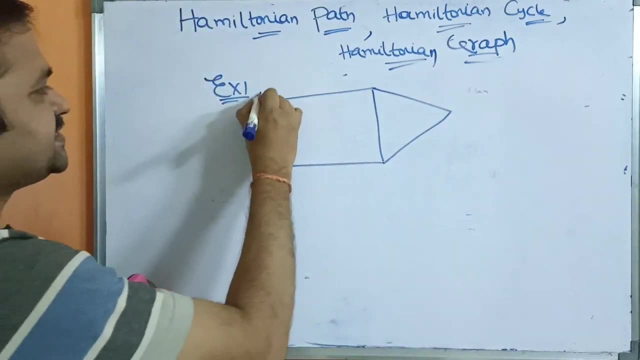 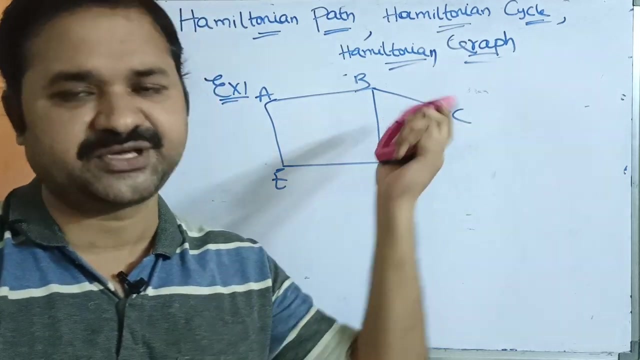 Let us see two examples regarding Hamiltonian graph or Hamiltonian circuit. This is the first example. We have a graph like this. Let the vertices are like this: A, B, C, D, E. We know what is Hamiltonian circuit. 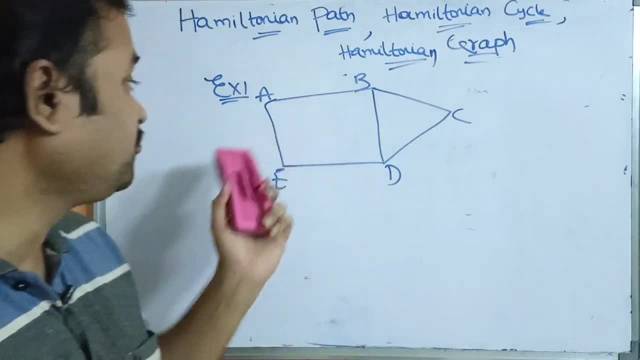 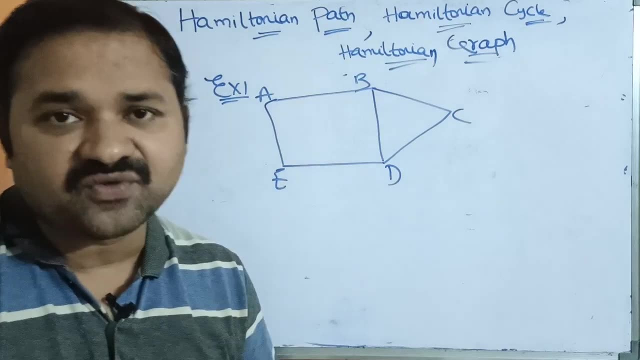 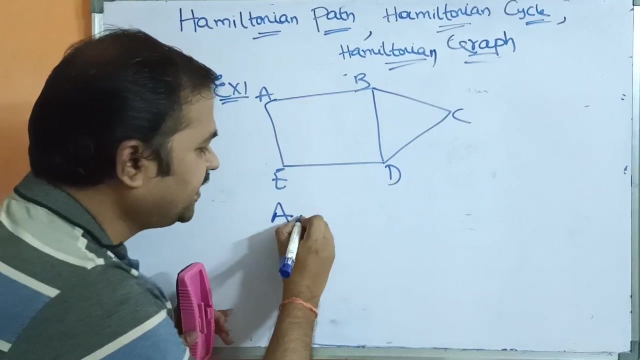 What is Hamiltonian circuit? We have to start at a particular vertex And we need to visit all the vertices of the graph And once again, we have to visit the starting vertex. Let here we have started at the vertex A, Okay, And then visit. 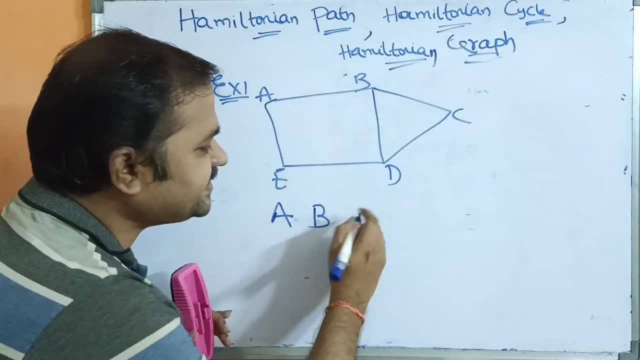 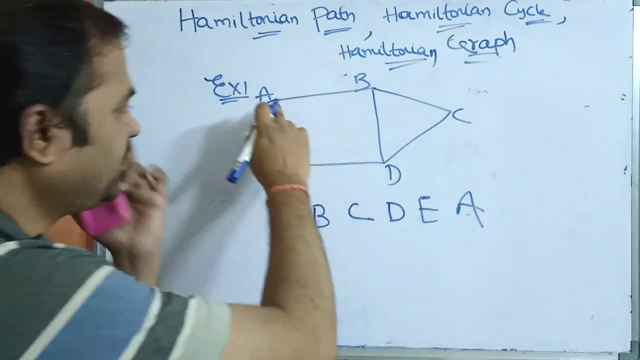 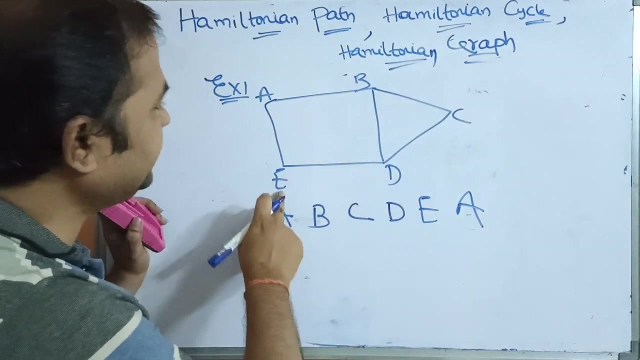 And then visit B, Then visit C, Then visit D, Then visit E, Then visit A. So here we have started at vertex A, Then visited B, Then visited C, Then visited D, Then visited E And then visited A. 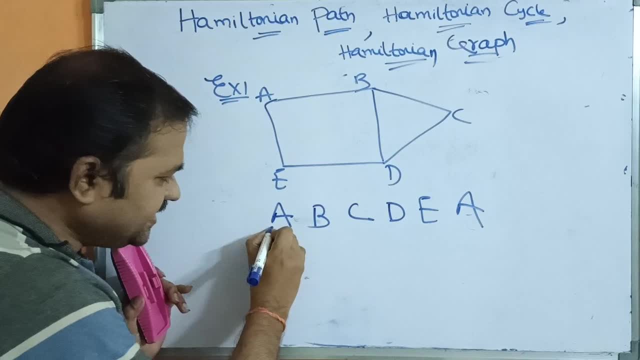 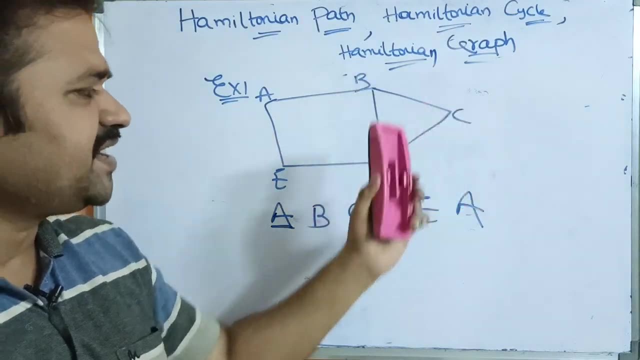 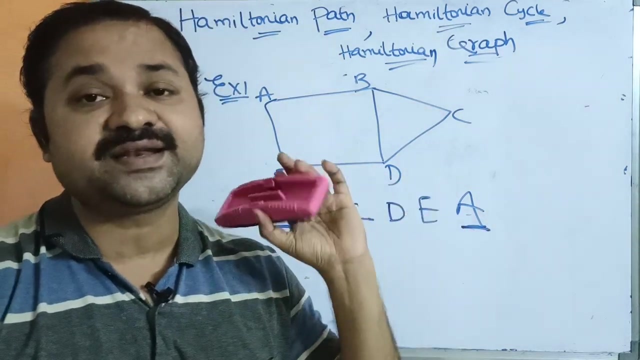 If we consider this cycle Here, the cycle is starting at vertex A And then visited all the vertices of the graph. What are the remaining vertices of the graph? B, C, D, E? And then visited the starting vertex. So this is called as Hamiltonian cycle or Hamiltonian circuit. 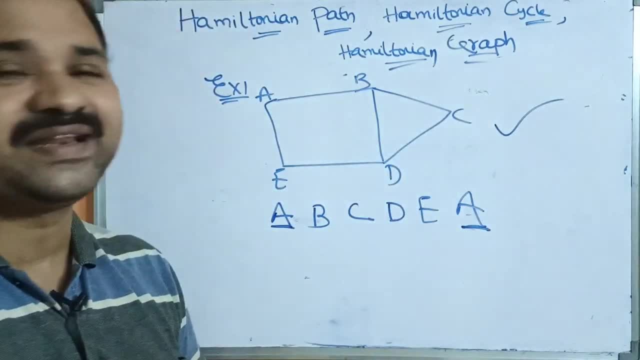 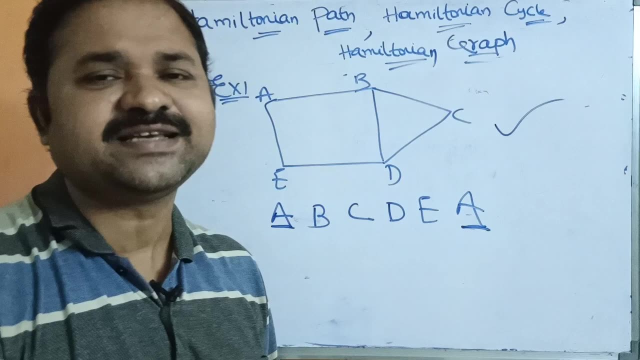 So we can say that this graph is Hamiltonian graph. Why? because what is Hamiltonian graph? If the graph contains Hamiltonian circuit, then it is called as Hamiltonian graph. ok, Here we have Hamiltonian circuit, So we can say that this. 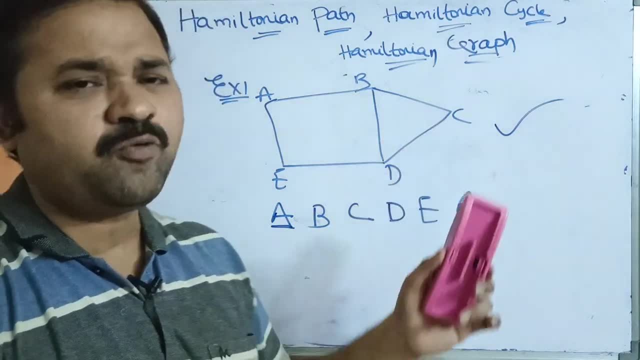 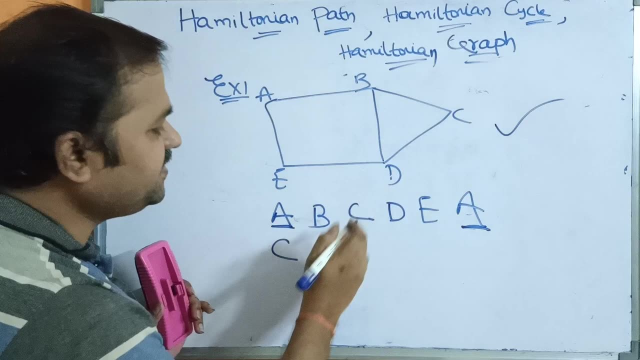 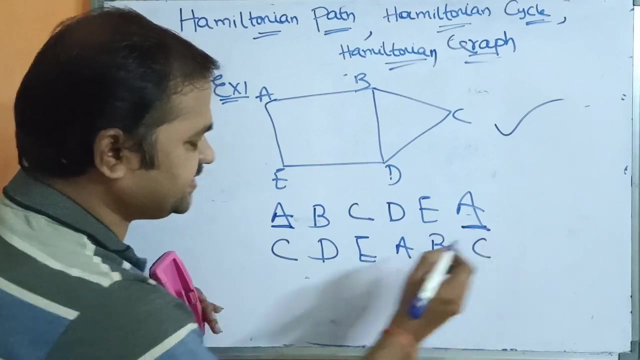 graph is Hamiltonian graph. Here a graph may contain several Hamiltonian circuits. ok, Let us start at the vertex C and then visit D, and then visit E, and then visit A, and then visit B and then visit C. Here, what is the starting vertex? C is the starting vertex and remaining 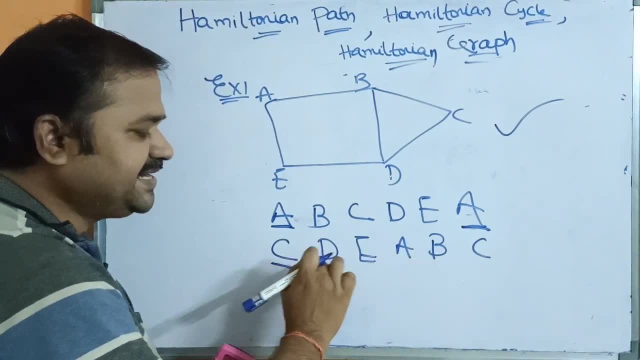 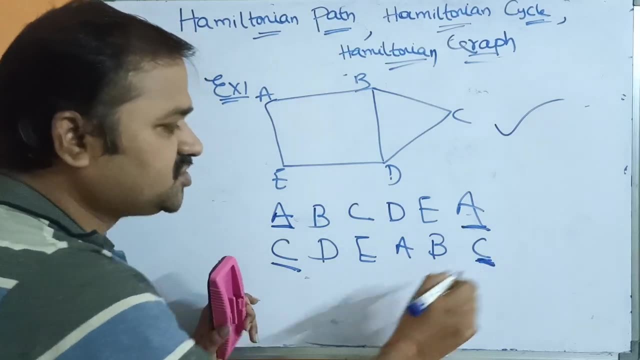 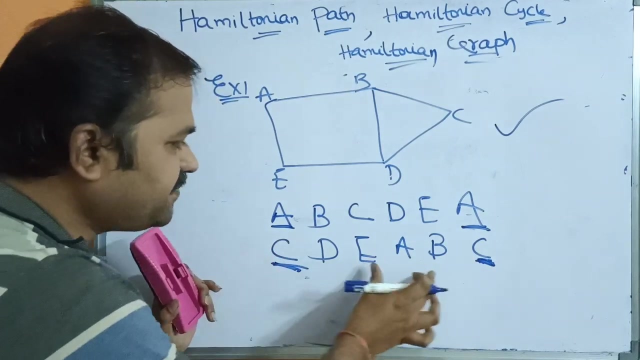 all vertices are visited: A, B, D, E. remaining four vertices are visited. and then we have visited starting vertex. ok, and then we have visited starting vertex. That means here the start vertex and the end vertex are the same and remaining all the vertices are visited. So 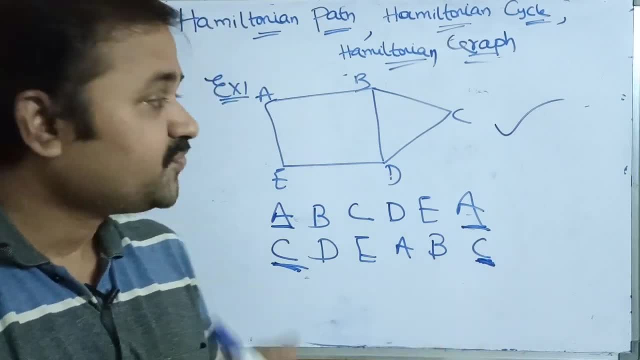 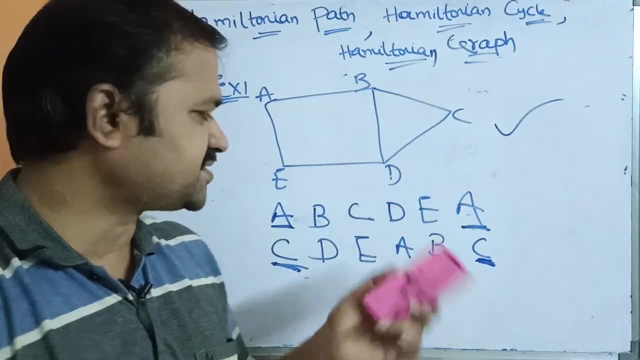 we can say that this is nothing but Hamiltonian cycle, So we can call this graph as Hamiltonian graph. A graph may contain several circuits, So out of all the circuits, if we draw, if we write one circuit, then that is enough. ok, Now let us see one more.